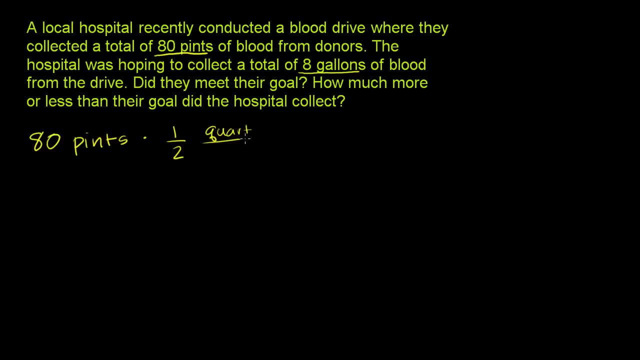 We have 1 quart for every 2 pints, Or you could view this as 2 pints per quart or 1 half of a quart per pint. Either way, The units work out And you're essentially taking 80 and dividing by 2 or multiplying by 1 half. 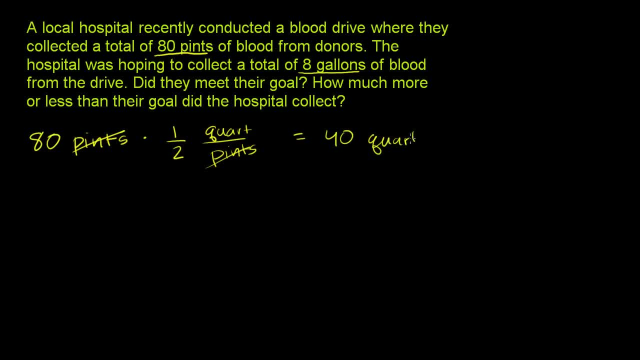 And you get 40 quarts. And I want to make sure that your brain does it both ways, Because when you're just doing it, you don't have paper, You don't have the units around. You should just think you know, hey, 80 pints. 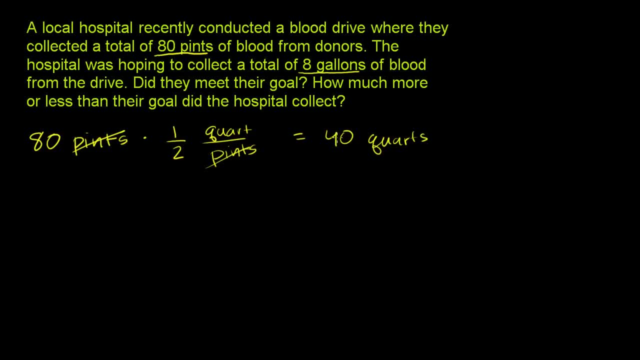 There's 2 pints per quart. I'm going to have half as many quarts. I'm going to have 40 quarts. But when problems get a little more complicated, it is nice to make sure that the units cancel out in this way. 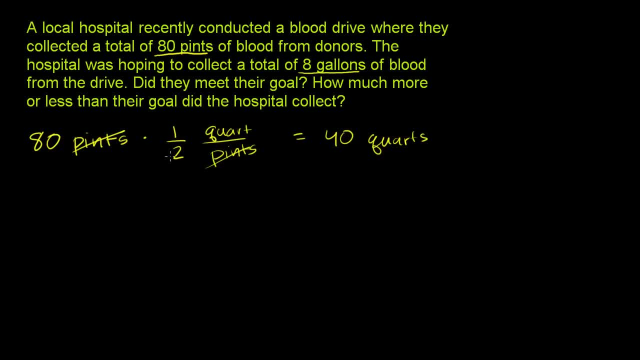 So that you know, OK, 1 quart is 2 pints- Pints in the denominator, Pints in the numerator. Cancel them out. I just left with quarts and 80 times 1 half, which is 40.. 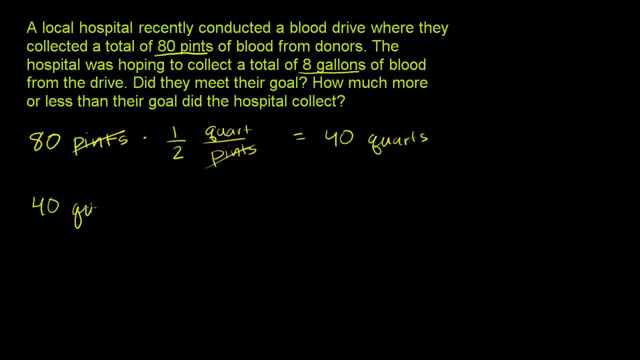 So we have 40 quarts now, And now we can convert this to gallons. We know that there are 4 quarts per gallon, Or that 1 gallon has 4 quarts, And once again we're going to go from a smaller unit. to a larger unit, to gallons. So we know there's a factor of 4 difference. Since you're going to a larger unit, your brain should say, hey, I'm going to divide by 4.. I'm going to have a factor of 4: fewer gallons. 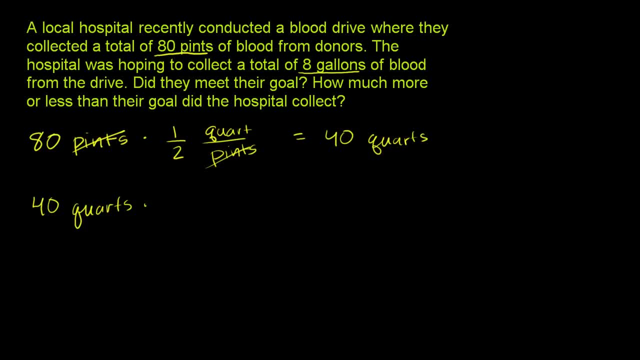 because it's a larger unit And to make sure that units work out. you just remember well, we have a quart up here in the numerator. You're going to want a quart down here in the denominator And we care about converting into gallons. 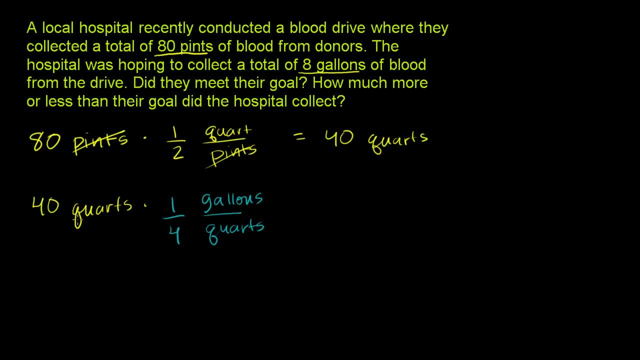 And 1 gallon is 4 quarts And this will work out. The quarts will cancel out And notice you're also dividing by 4.. 40 times 1 fourth is the exact same thing as 40 divided by 4, which makes sense. 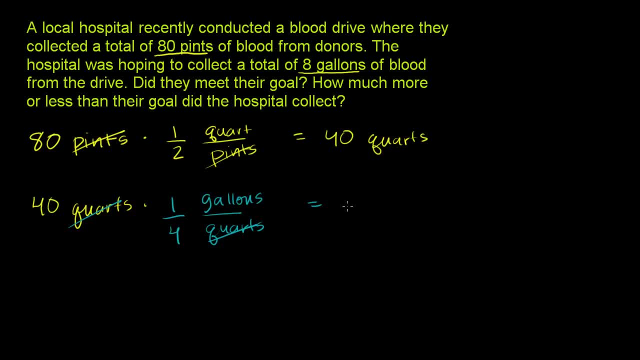 We're going to a larger unit, So 40 times 1 fourth. 1 fourth is 10.. And the units left are gallons. So the 80 pints of blood that the hospital collected is 10 gallons. Their goal was only 8 gallons. 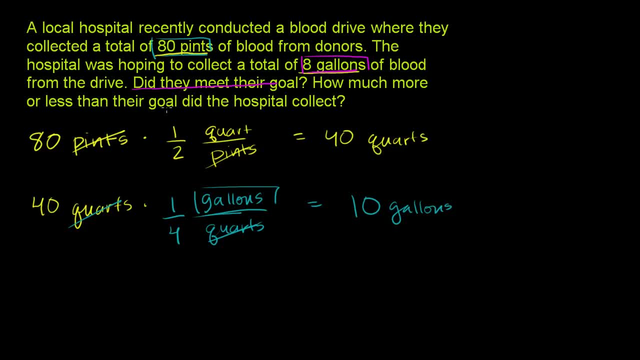 So did they meet their goal? Yes, they met their goal. How much more or less than their goal did the hospital collect? Well, their goal was 8.. They collected 10.. They collected 2 extra gallons- Their goal.